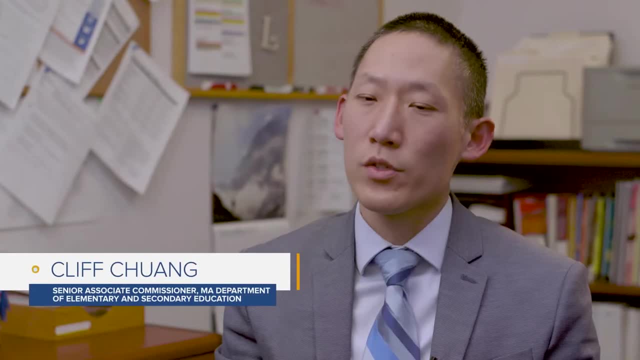 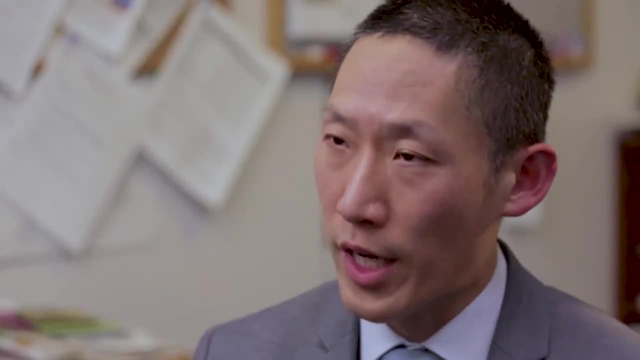 students. Where do we want them to be? We want to make sure all of our students are really prepared for the jobs and careers that the 21st century has to offer and what our world needs, and our new standards are really supporting the development of students in terms of their skills that can really be applied. 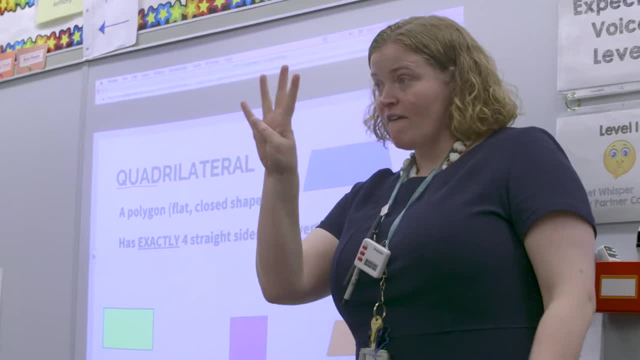 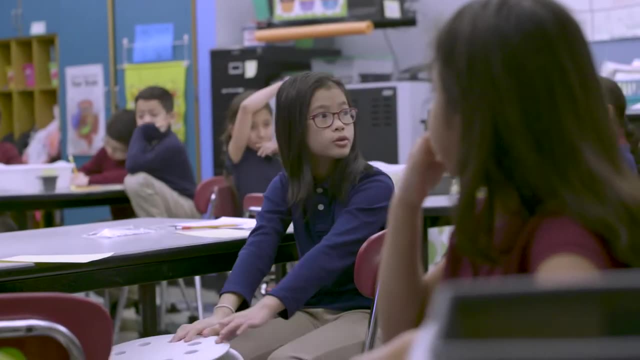 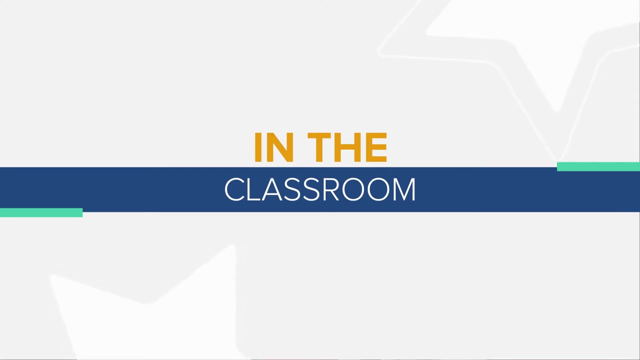 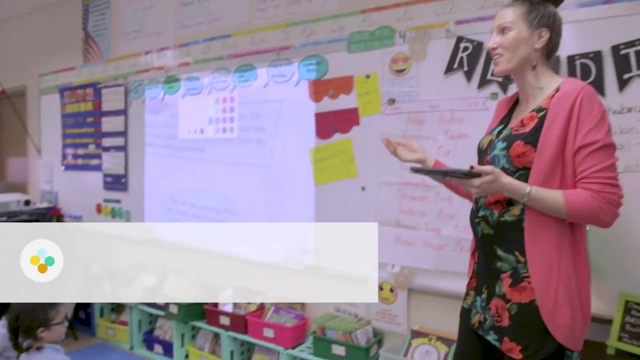 in the workplace. Our hope with these standards is that the students will take the knowledge and skills learned in the classroom and take it beyond the there, for instance in everyday life and society. Students in mathematics should engage with meaningful real-world problems every single day. Teaching math has real-world problems, not just as numbers. 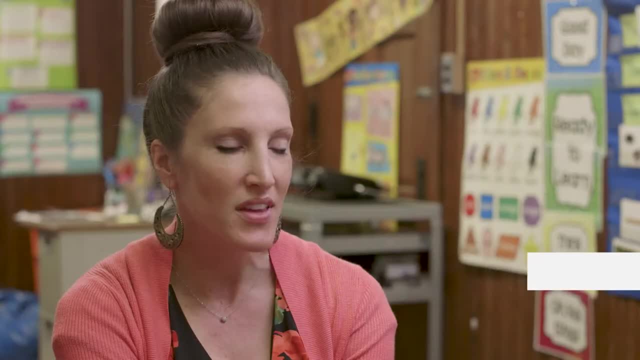 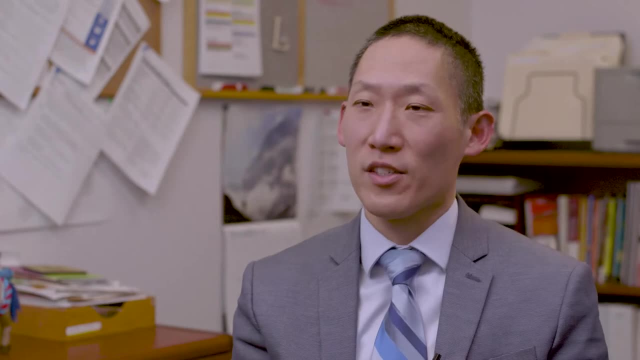 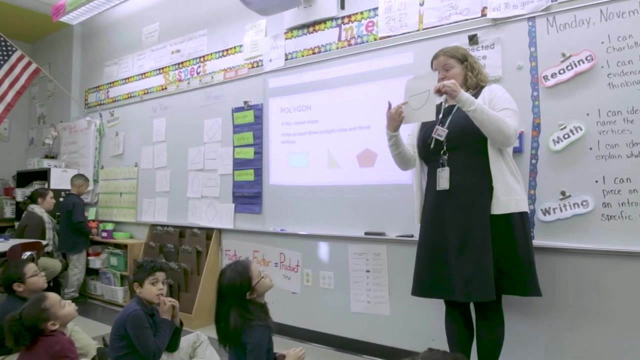 It sets them up to look at a problem that they're facing and have skills, have a toolbox of strategies they've used to solve something before. The way that they learn best is if they're really actively, sort of involved in the learning process and really seeing how it applies to their own lives and our. 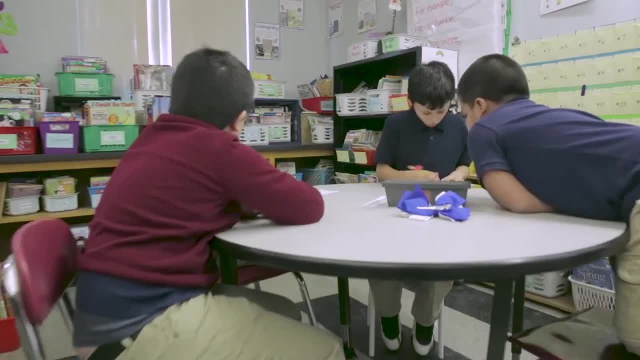 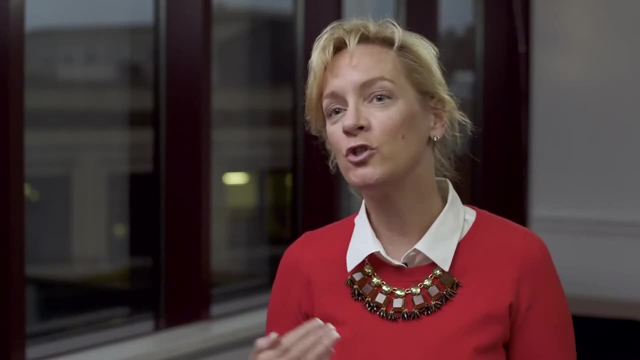 new standards are really designed to make sure that students are grappling with real stuff. I need to have the carpeting fit the room. I need to figure out the tip for my restaurant bill For children. they need to understand that math is really a part of real-world life and is a way that we solve problems as 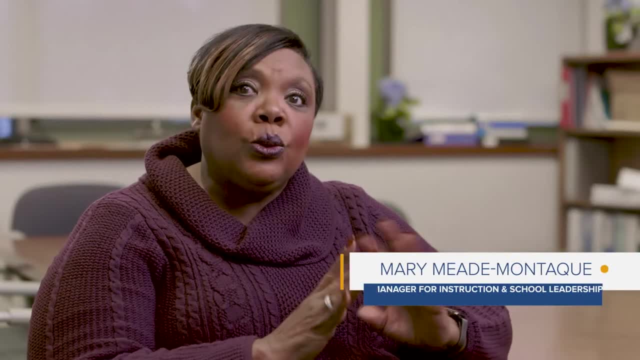 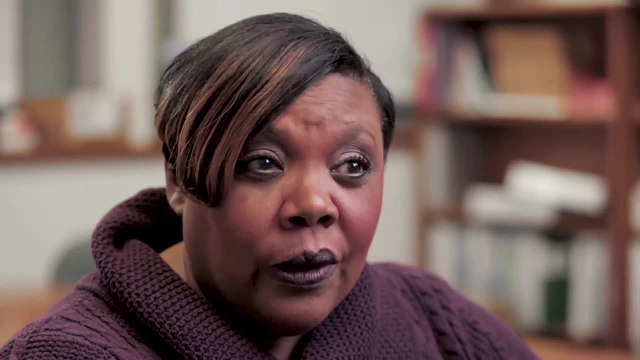 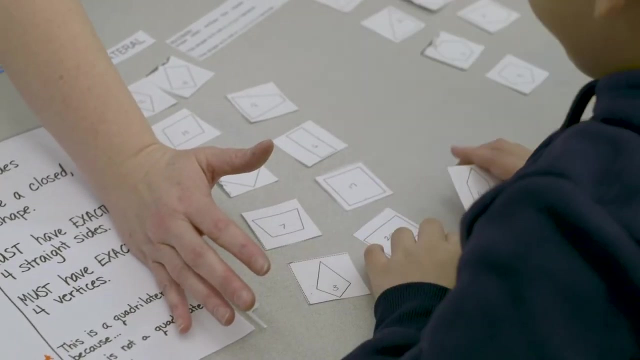 children and, of course, as adults too, Once you learn the things that they've valued and the things that they do every day and become a part of their world. that way you're able to develop real-world problems that relate, that are relevant to their everyday life, If I come up with this great problem, but the 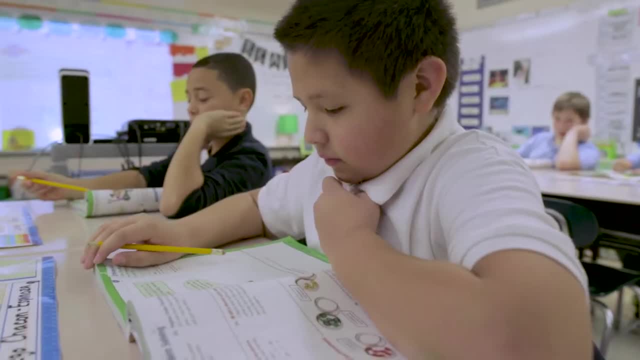 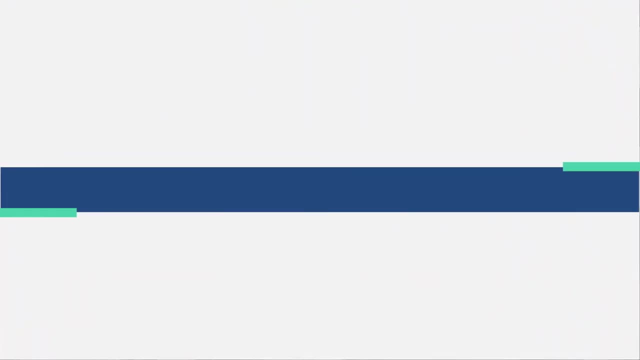 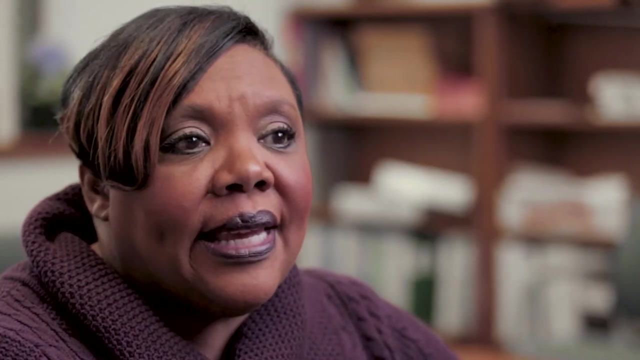 students have no idea the background of the problem. that real-world problem will actually get in the way of them understanding the mathematics. Music, Music, Music, Music, Music is around being able to take academic risk. If we stay safe, we don't learn as much. 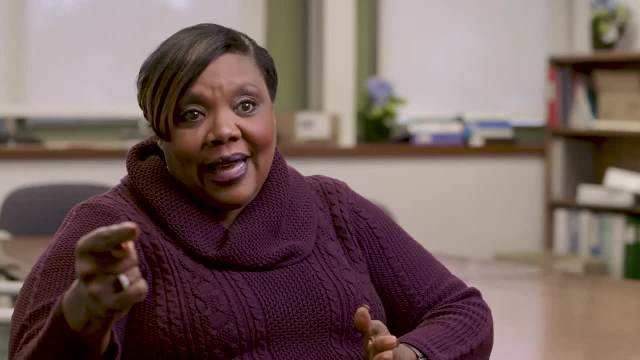 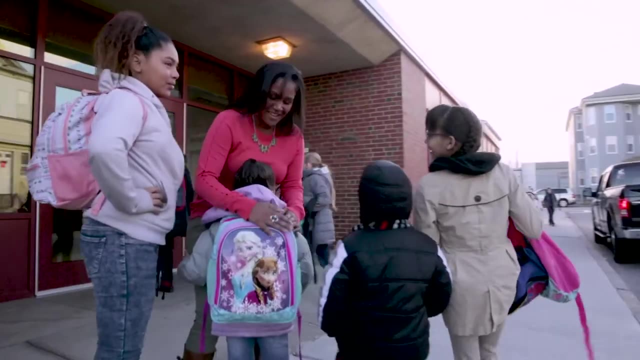 You have to be able to go beyond, to be able to look at that next step, which is really about confidence. The kids need the academic skills that we teach through the standards, but they also need the soft people skills that just make you a nice whole person.